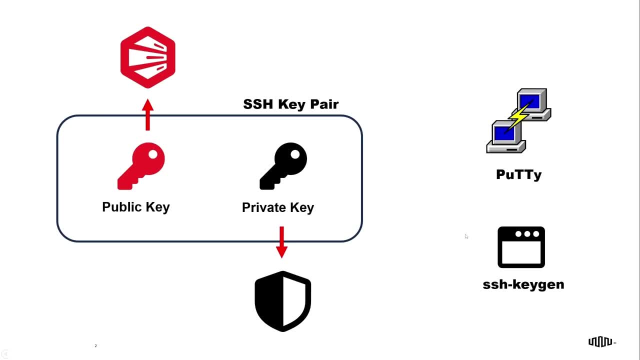 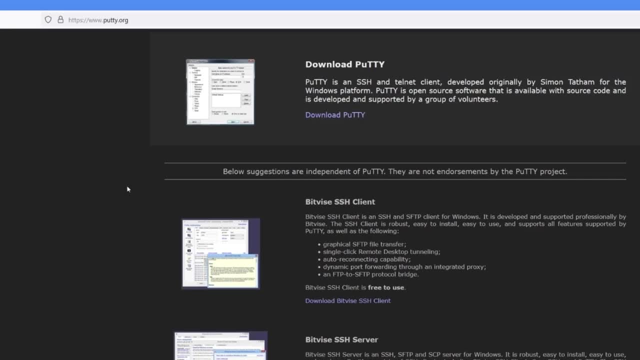 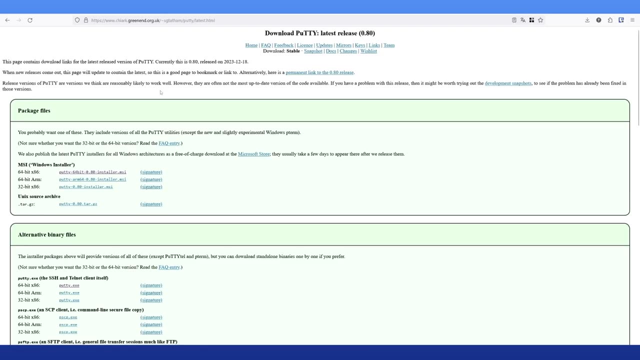 SSH keygen which can be used on Windows or any Unix-like systems. So let's start with PuTTY. To download PuTTY, you can access the PuTTYorg website and when clicking on this link here, it will take you to a website with different versions and installers. 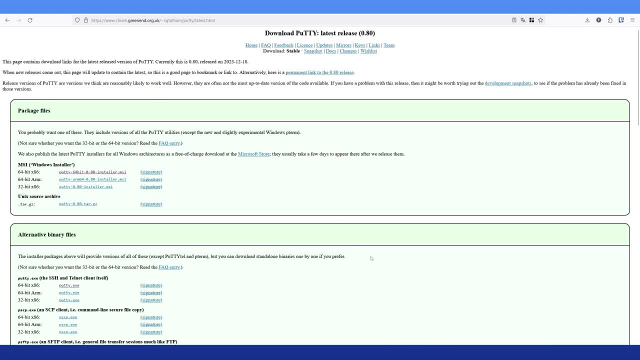 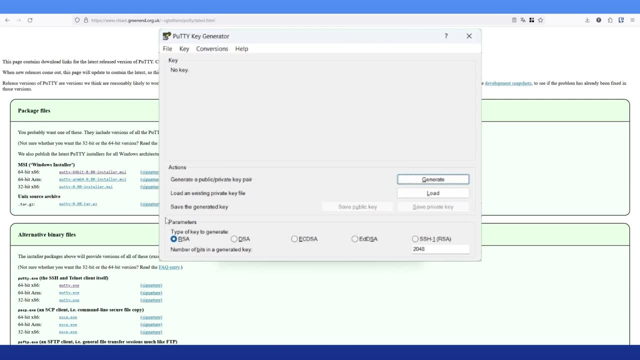 for different OSs. Once you have it installed, this is what you have. It's just a PuTTY key generator which has not done many configs, and for Equinix Metal you can keep the type of key to generate as RSA. 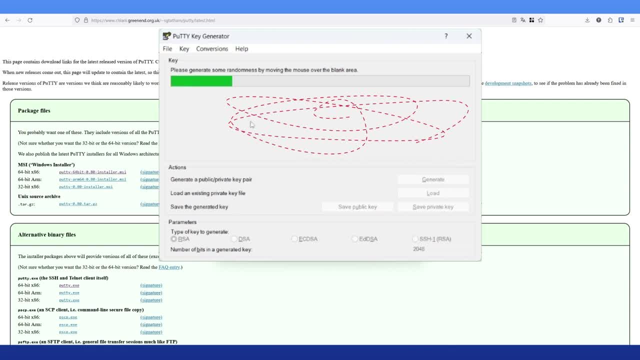 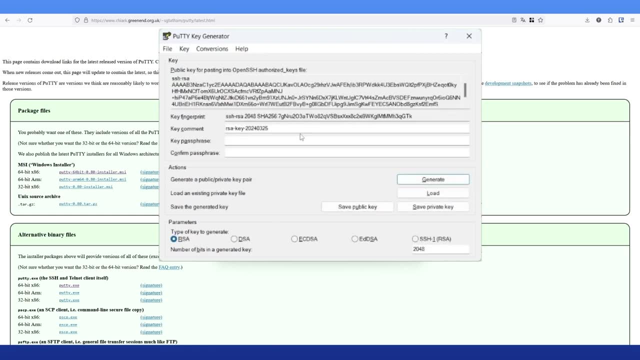 So when clicking generate, it will ask you to move the mouse over this blank area for a second, and by doing that, here you go. you have the public key. We recommend that you copy and paste this public key here directly to your PC. 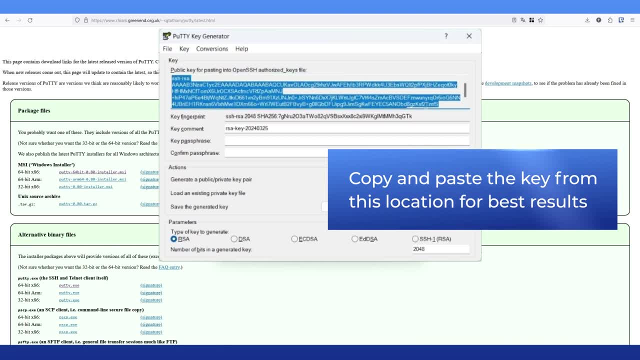 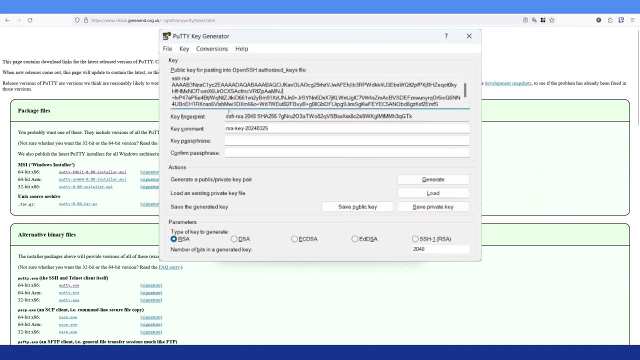 To the Equinix Metal console. this way, you'll make sure that your pair of public and private key are working properly. After copying and pasting the public key onto the Metal console, you can save your private key by pressing this button. It will ask you if you want to save this key without a passphrase. 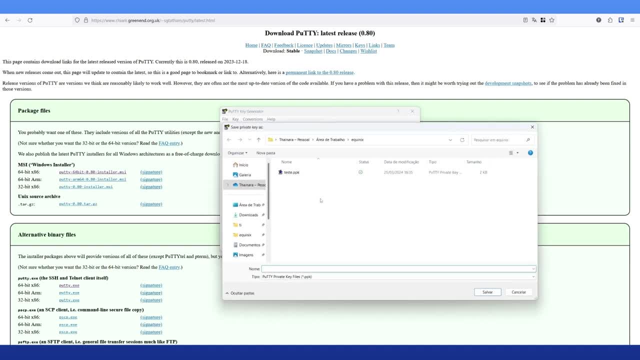 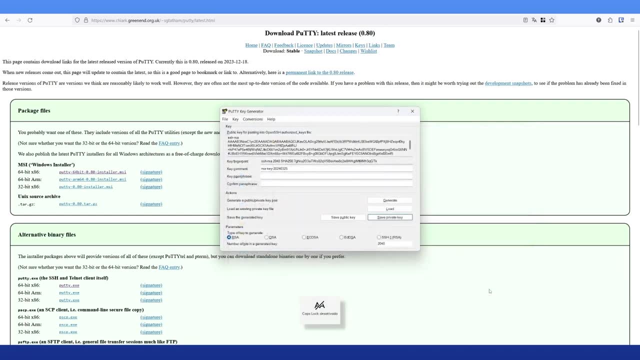 which is what I'll do. I'll just click yes and I'll save it with the name test key. Once it's saved, I'll be able to use it to access my Equinix Metal instance alongside with the public key that I already pasted on the Metal console. 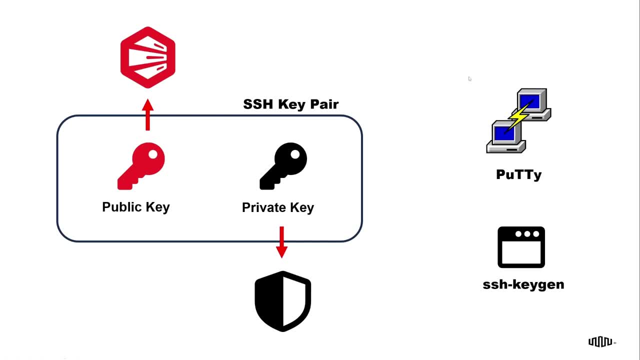 Now that we learned how to create the SSH key by using PuTTY, let's do the same thing, but this time using the SSH key gen application that you can find on whatever terminal you want on your preferred OS. Here I'm going to use a Linux system to show. 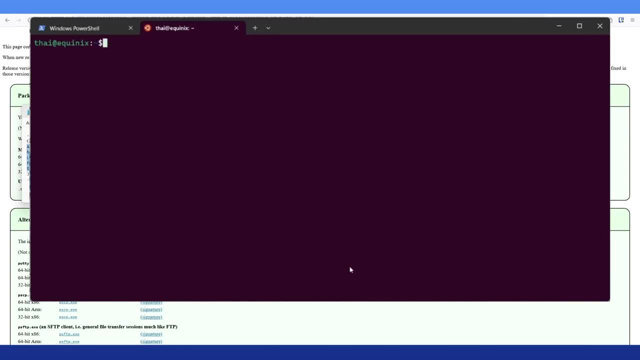 Uh, it is a very simple command. You just type ssh-keygen and when hitting enter, it will generate the public key pair and it's going to ask you for a file in which you saved the key. If you press enter, it's going to save in this directory. that is showing. I'm just going. 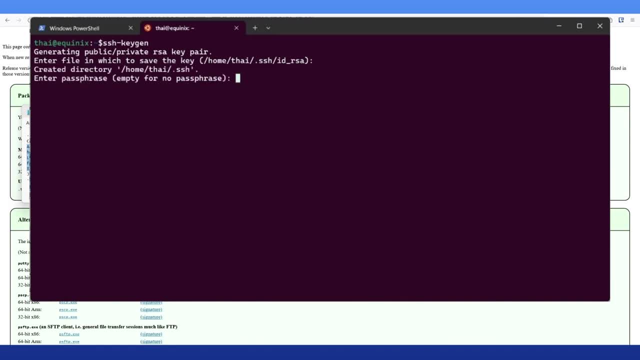 to press enter, It's going to ask for a passphrase Again. I'm not going to use one, so I'm just going to hit enter Again. it asks for the same passphrase again. so just enter again, and there you have it. 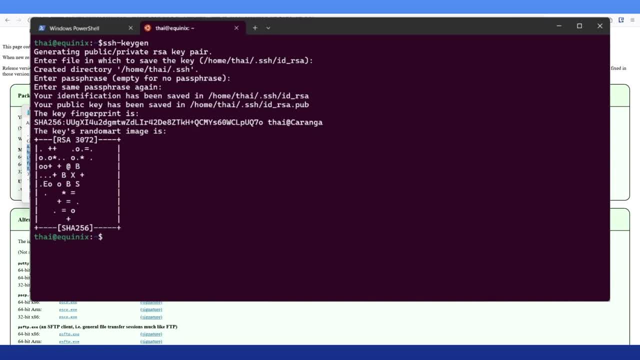 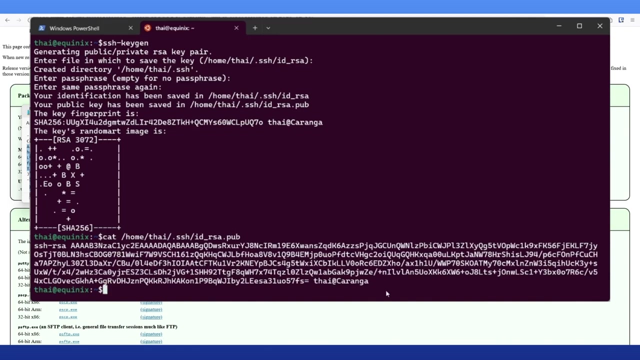 To copy it and paste it onto the Equinix Metal console. I'm just going to do. I'm just going to print the public key here on the terminal And there you have it. I just pasted The public key on the terminal and now I can just copy and paste this onto the Equinix. 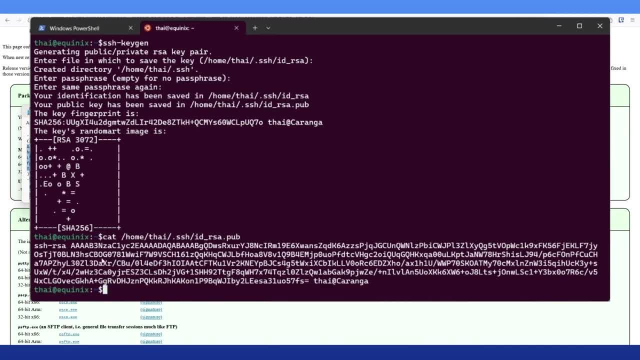 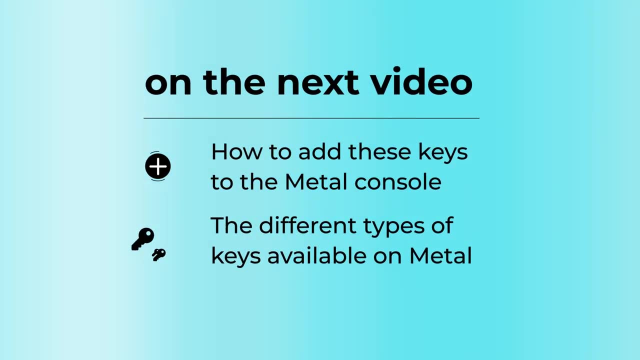 console website and there you have it. You have your key pair that has been generated on either Windows or Linux, And on the next video we're going to talk about how to add these keys to the Equinix Metal console and the different type of keys that you can have on Metal. 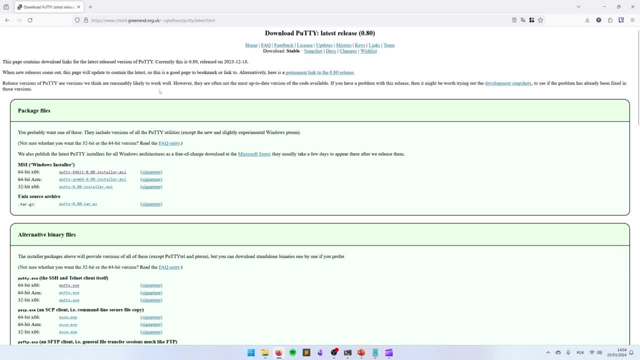 I hope this video helped you to create your keys. Thank you so much for watching and stay tuned for the next videos. 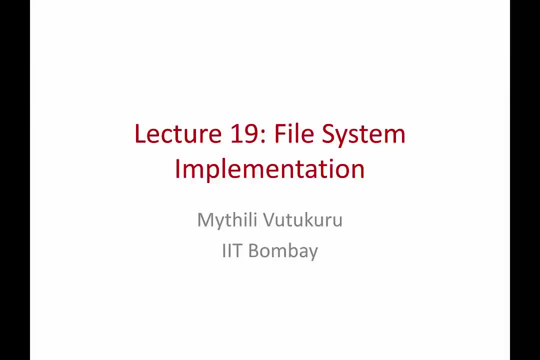 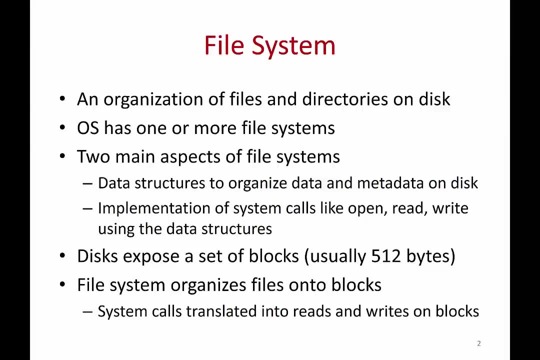 In this lecture we are going to study how various operations on files are implemented in a file system. So what is a file system? A file system is simply an organization, a way of organizing files and directories on disk right, So disks.